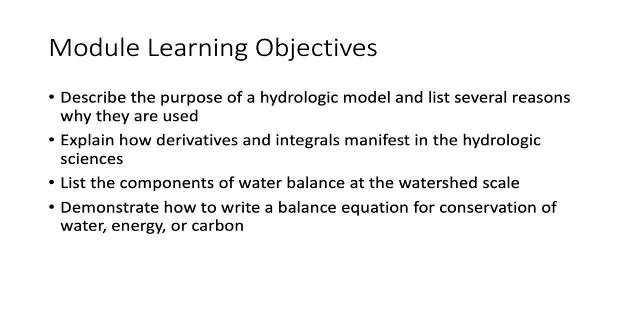 A little bit about explaining how derivatives and integrals might manifest in the hydrologic sciences, listing the components of the water balance at the watershed scale. That's going to be critical. in this module, We're going to be talking about how to write a balance equation for water conservation, designing our model and demonstrating how to write a balance equation for conservation of water in particular. 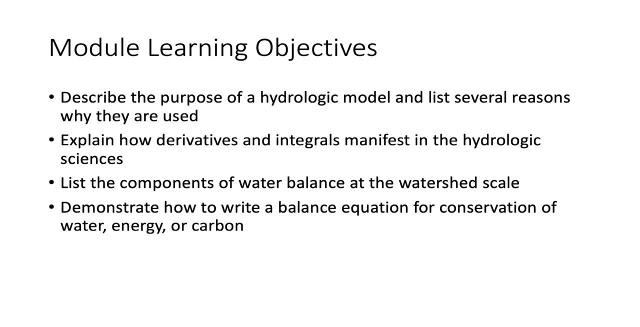 So when I teach a whole class about modeling, I spend maybe the first lecture going over sort of a philosophical discussion of what a model is, And what I found over the years is that the easiest way of actually doing that is to just start off with a simple example. 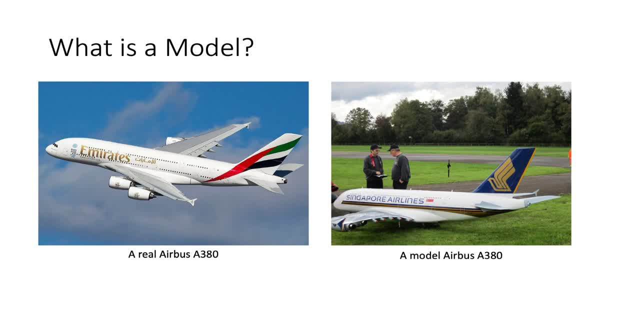 Okay, so what is a model? So here is a contrast in the comparison between what a model is and the actual underlying thing that that model is seeking to replicate. So on the left-hand side, here we have a real Airbus A380.. This is the giant double-decker long-range, long-haul aircraft developed by Airbus. 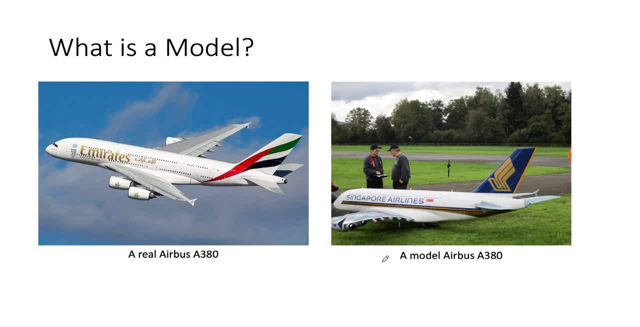 And on the right here we have a model of an Airbus A380.. This picture here is a model of an Airbus A380.. This picture here is a model of an Airbus A380.. This particular model is a radio-controlled model, meaning that it also flies, but it is sort of spatially scaled down from the actual Airbus A380.. 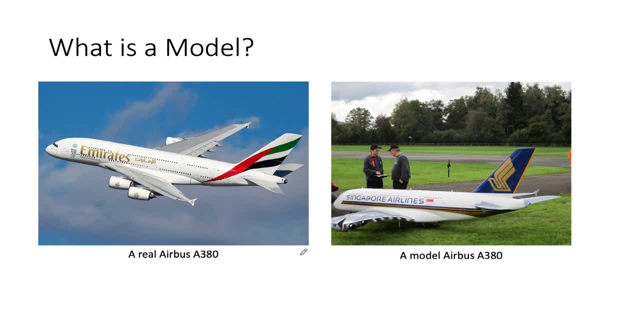